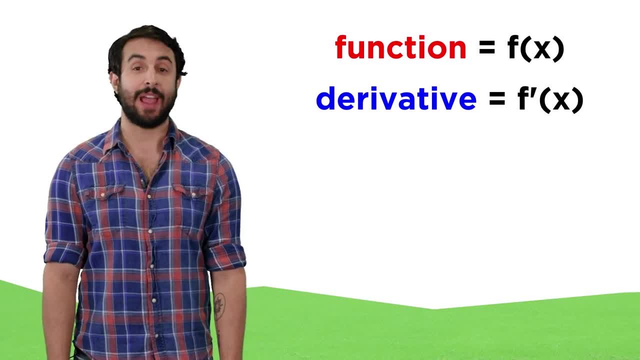 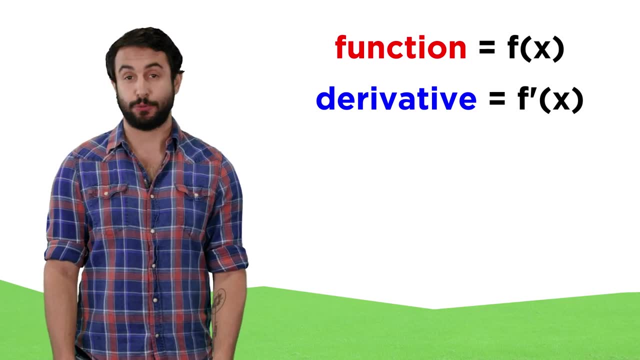 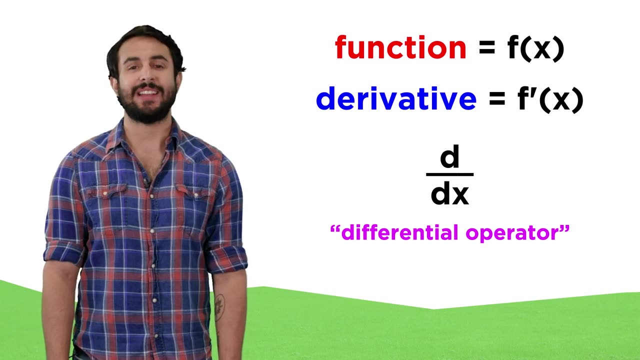 So the derivative of f of x was f, prime of x. But there is another notation which we have introduced in the past that will now be used much more frequently, That looks like this, which is read: d, dx. This can be thought of as a differential operator that acts on whatever we put it in front of. 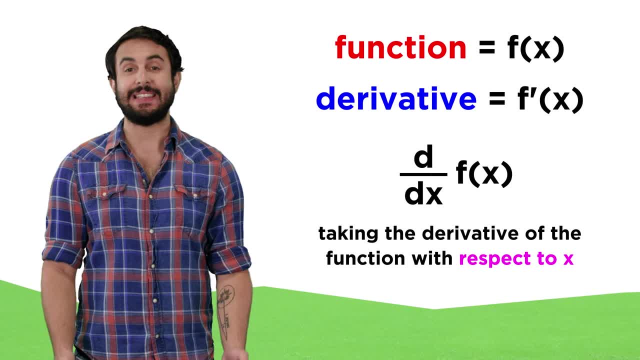 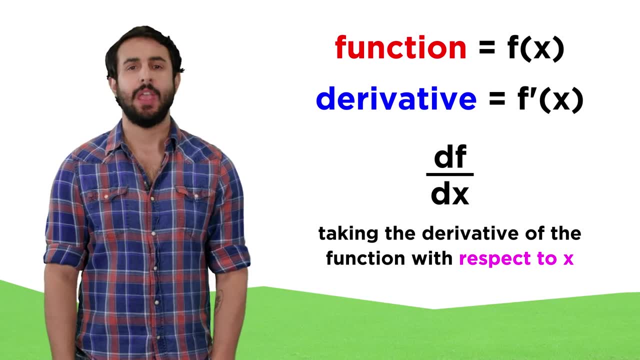 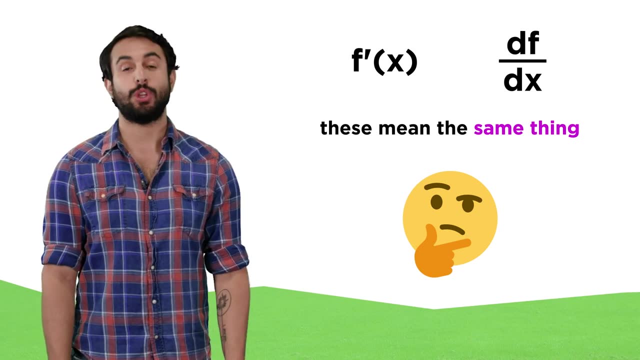 So, to take the derivative of f, we would put d dx in front of it, like so This is also commonly written as df dx. Now, don't let the new notation confuse you. This is still the same as the derivative of some function, f, which we previously called. 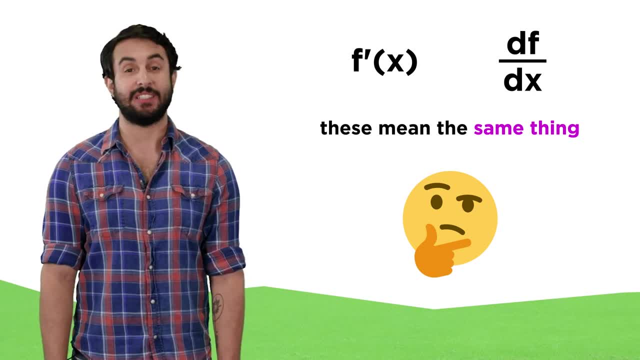 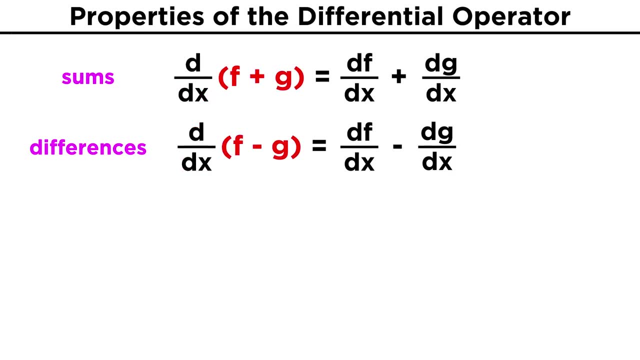 f prime. It's just a different way of representing differentiation that has a few benefits. For example, this differential operator distributes across sums and differences, so d- dx. of the sum of two functions, f prime, This is the same as the sum of df, dx and dg dx. 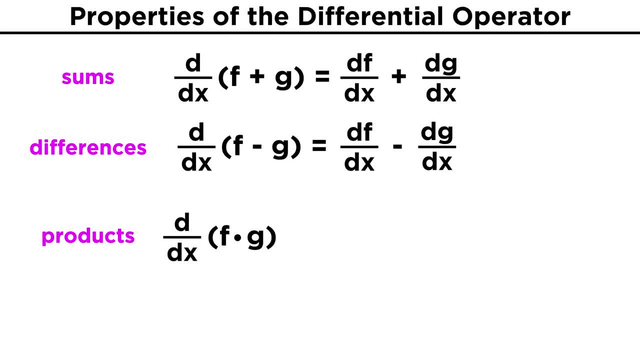 Meanwhile, when operating on a product of functions, f times g, this will be the same as the product rule we learned previously. so d dx f, g equals f, dg, dx plus df, dx g And similarly the quotient rule still applies: d dx f over g equals g, df, dx minus f, dg, dx over g squared. 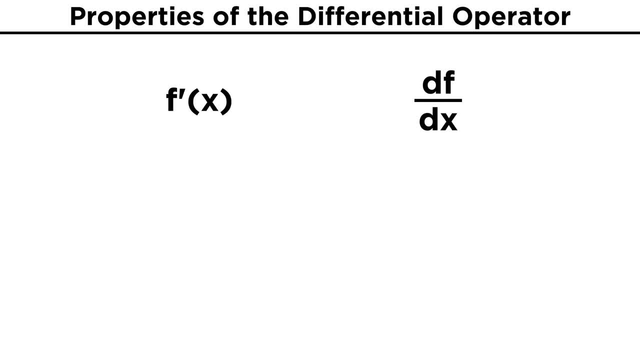 The reason we are reintroducing this notation now is because we will want to take more derivatives than just those that are with respect to the variable x. so we need some clear notation that indicates which variables are going to be in the variable x. So we need some clear notation that indicates which variables are going to be in the variable. 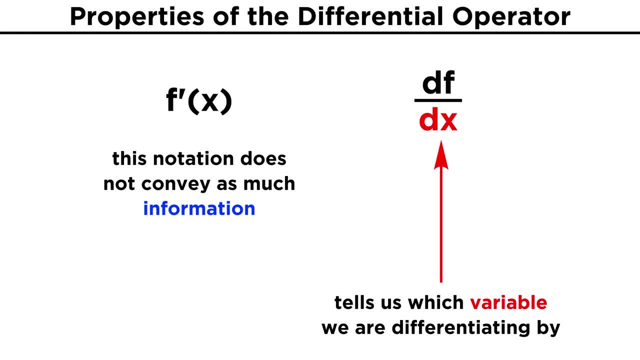 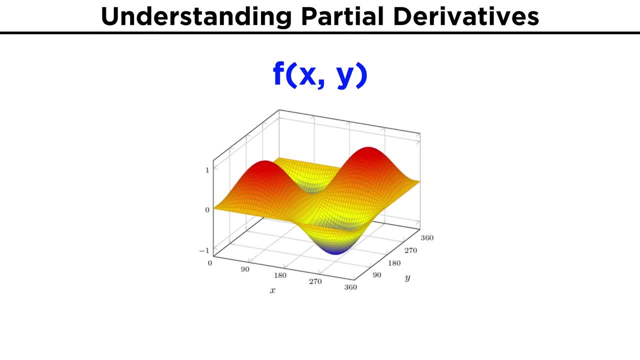 x. So we need some clear notation that indicates which variables are going to be in the variable y. Now let's say we have a function that depends on both x and y, which we can call f of xy. This will end up being a surface in space rather than a curve, so how can we interpret? 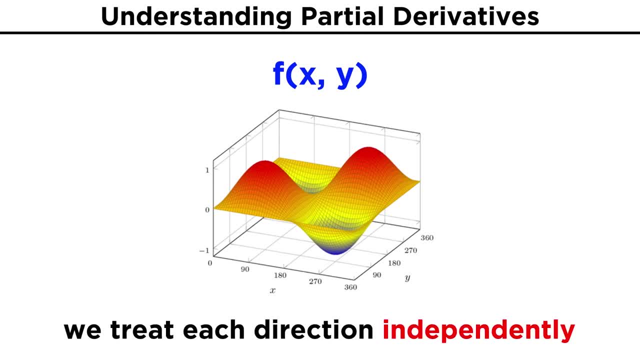 the rate of change. for this, What we end up having to do is to find the rate of change in specific directions independently. If we want the rate of change in the x direction, much like we have been doing already, we simply differentiate with respect to x, while treating y as a constant. 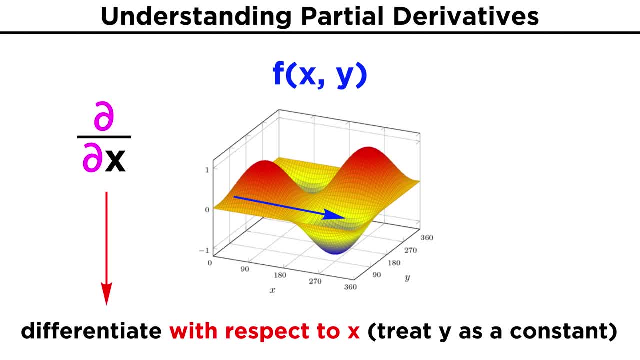 The new notation for this involves using these curvy d's instead of regular ones, which gives us this: This is called a partial derivative and it tells us to only treat x as the variable to differentiate. Similarly, if we wanted the rate of change in the y direction, this would be a partial 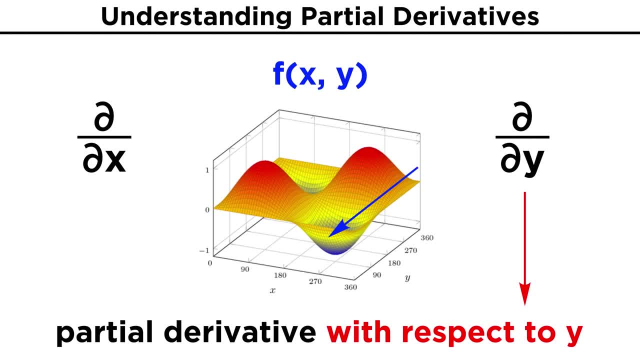 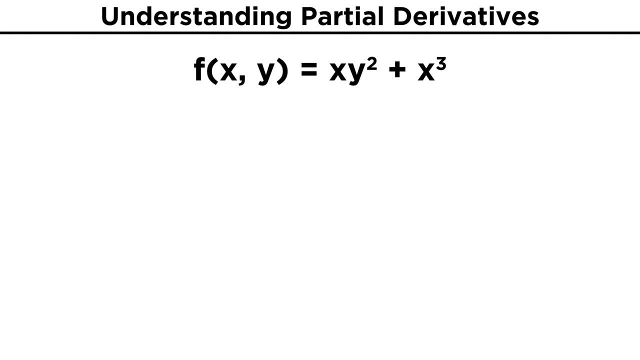 derivative with respect to y. In this case we would treat x as a constant. Let's consider an example: f of xy equals xy squared plus x cubed, and find the partial derivatives with respect to x and y First: df, dx. 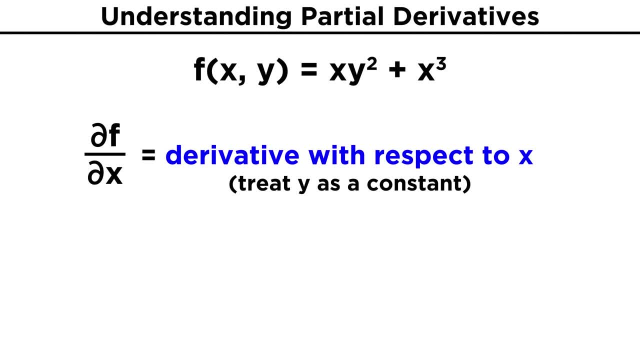 We will take the derivative with respect to x, just like we are used to, while treating y as a constant, Remembering our power rule for derivatives- the first term's x becomes one- and treating the y squared as a constant. we are just left with y squared. 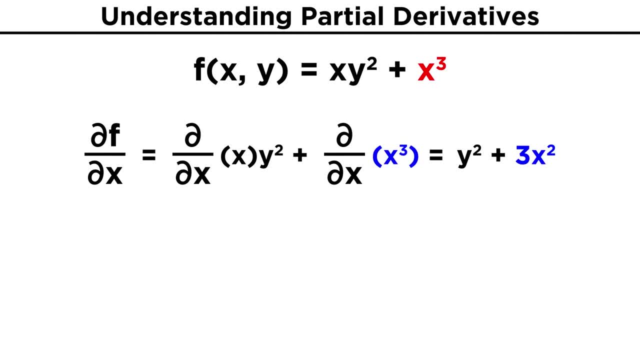 Then, for the second term, we bring down the three and reduce the power by one, leaving us with three x squared. So our partial derivative becomes one. The partial derivative df, dx becomes y squared plus three x squared. Now to find the partial derivative with respect to y, we will treat y as our variable, while 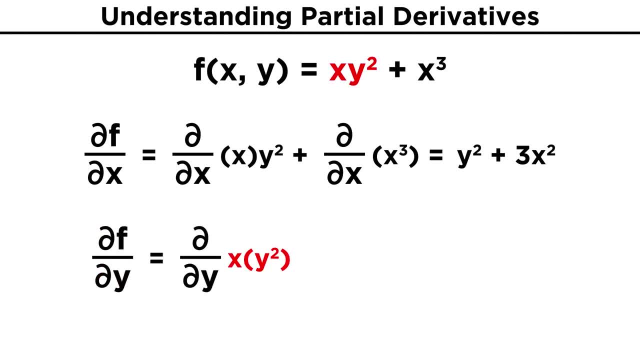 treating x as a constant. The first term depends on y squared, so we bring down the two and reduce the power by one, leaving us with two y. But this is multiplied by x, which we treat as a constant. So we get two x- y. 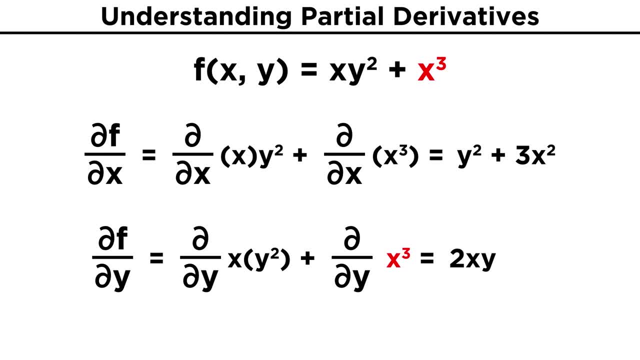 The second term does not depend on y, so this is just a constant and the derivative of a constant is always zero. So we are left with two x- y for our partial derivative, df, dy. These are the rates of change in the x and y directions for our function. 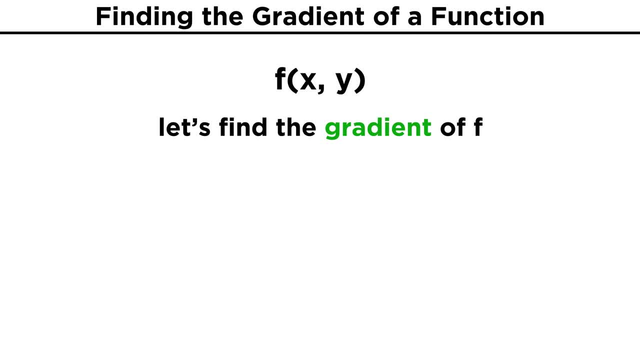 We will now introduce a concept that combines these partial derivatives. We will now introduce a concept that combines these partial derivatives. We will now introduce a concept that combines these partial derivatives, derivatives, and that is called the gradient. The gradient of a function is simply a vector made up of all its partial derivatives. in 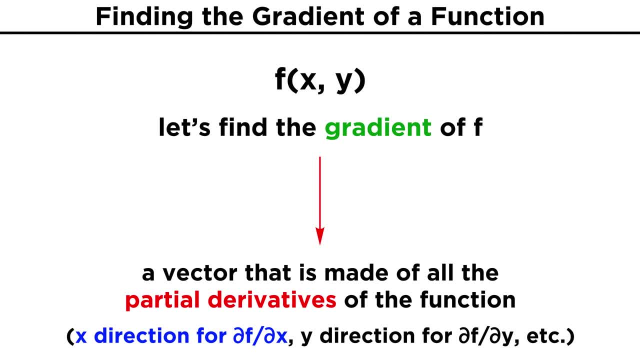 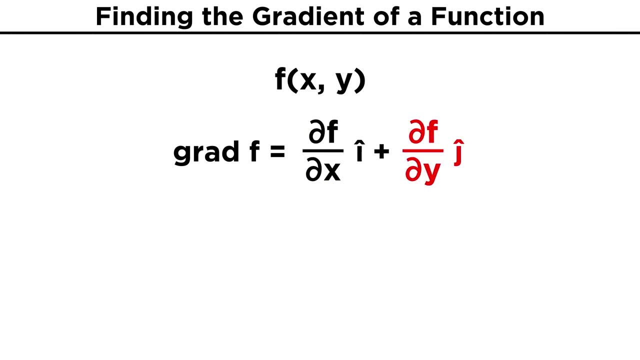 their associated positions. This means the X direction for DFDX, the Y direction for DFDY, and so on. We can write this out as grad F equals DFDXI plus DFDYJ. If in three dimensions that would be grad F equals DFDXI plus DFDYJ plus DFDZK. 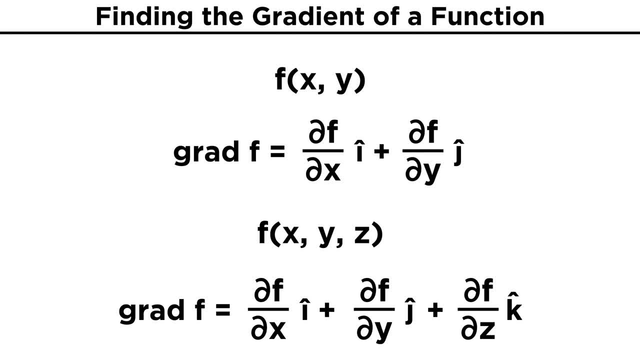 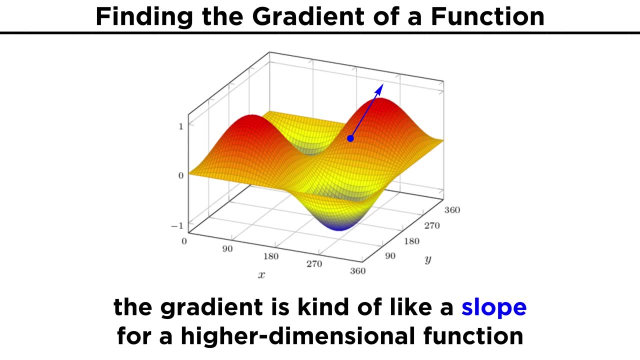 The components of this gradient vector are the partial derivatives of the function F, which we can think of as the gradient vector. This vector ends up being the closest thing to a slope that we can get in higher dimensions. It points in the direction of maximum change of the function and has a magnitude equal. 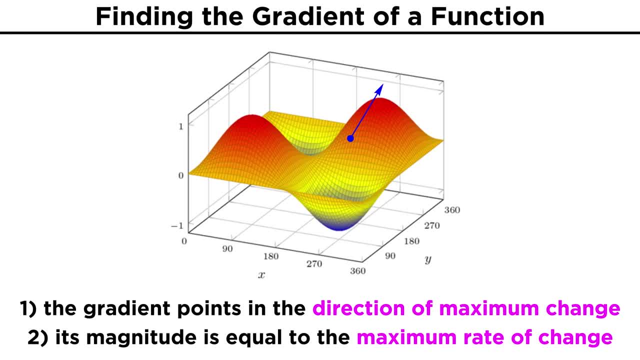 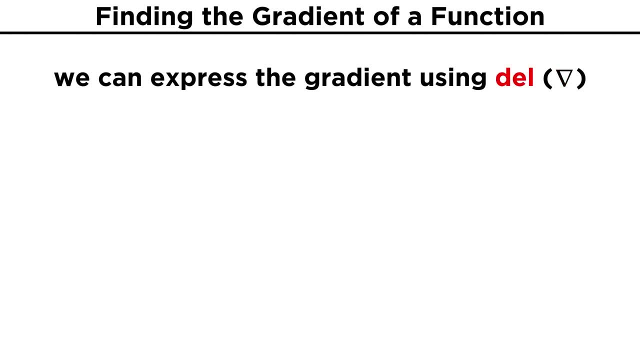 to the maximum rate of change. There's also another common way to write the gradient involving this upside-down triangle, which is referred to as DFDX. It's called a del. This del is a vector of all the partial derivative operators, so in two dimensions it is DDXDDY. 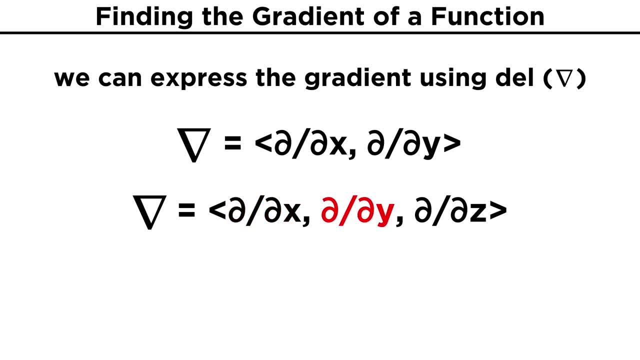 and in three dimensions it is DDXDDYDDZ. Writing del in front of a function F is the same as taking its gradient. Del has a variety of other uses that we will get into in another lesson, but for now let's. 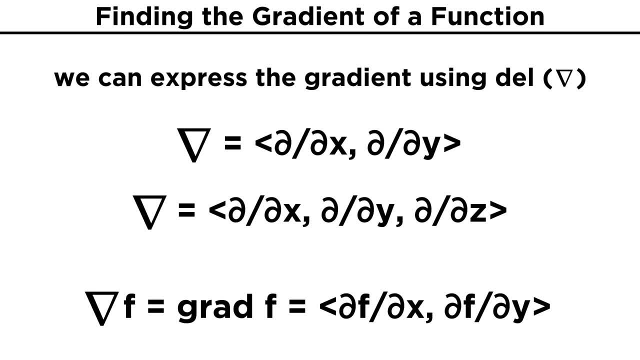 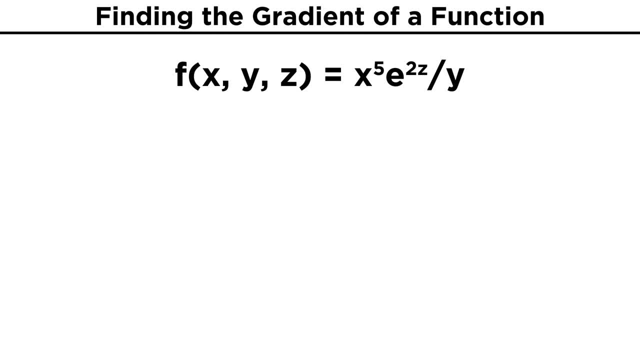 consider one more example. Let's take a look. Let's take a look at the example of a function and find its gradient. Consider the function F of XYZ equals X to the fifth E to the two Z over Y. To find the gradient we will need all the partial derivatives DFDX, DFDY and DFDZ. 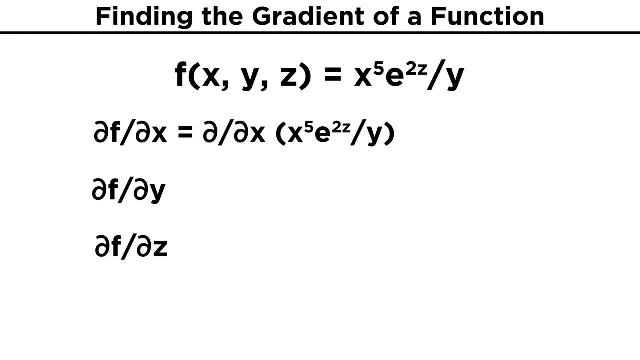 Starting with X and treating Y and Z as constants. following the power rule, we bring down the five and subtract one from the exponent, leaving us with five X to the fourth, E to the two, Z over Y for our partial derivative with respect to X. 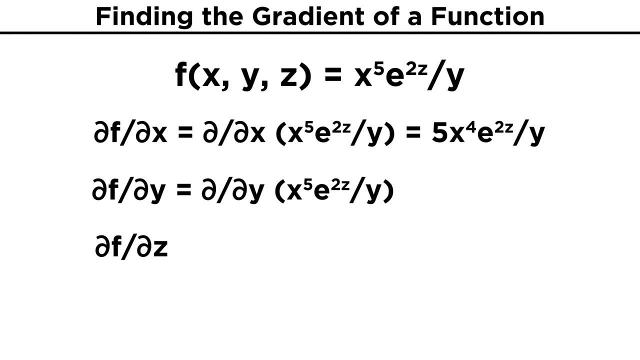 Now differentiating with respect to Y and keeping X and Z constant. one over Y is the same as Y to the negative one. So, again, using the power rule, we bring the negative one out front and subtract one from the exponent to get negative Y to the negative two, which is the same thing as negative one. 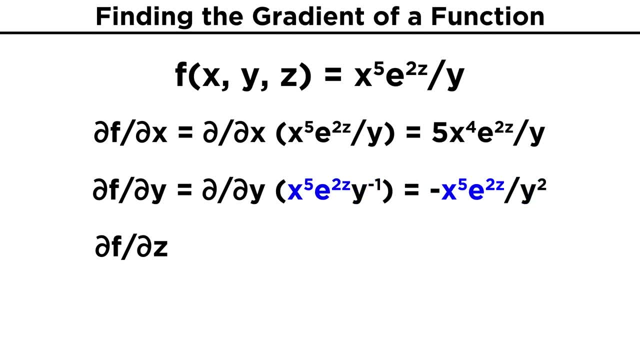 over Y squared. Combining this with the constant terms, we get negative: X to the fifth, E to the two, Z over Y squared. Finally, we will take the derivative with respect to Z. while keeping X and Y constant, We must differentiate E to the two Z and, following the chain rule, we get negative. 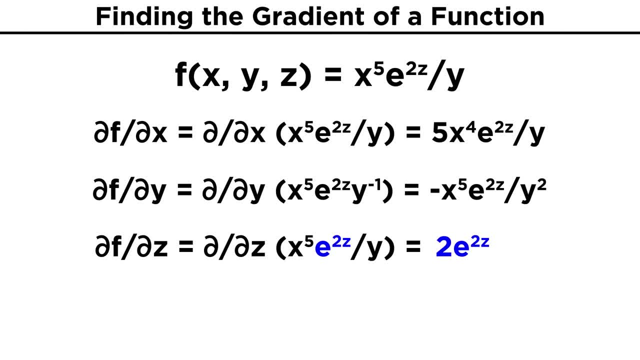 X to the fifth, E to the two Z over Y for our partial derivative with respect to Y. So, again, using the power rule, we simply keep the E to the two Z, but bring down the derivative of the exponent two Z, which is two. 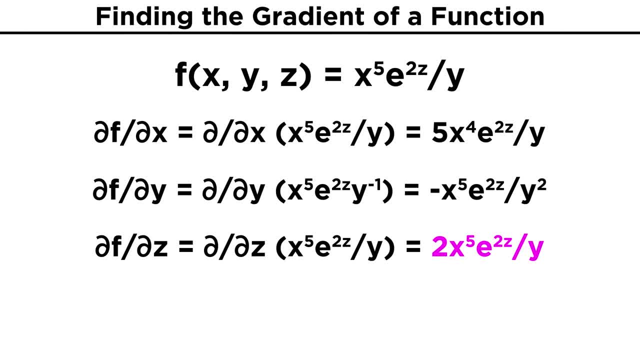 This gives us two E to the two Z and putting it together with the constant terms, we get two X to the fifth, E to the two Z over Y. We now have all three partial derivatives. This gives us five X to the fourth, E to the two Z over Y, negative X to the fifth. 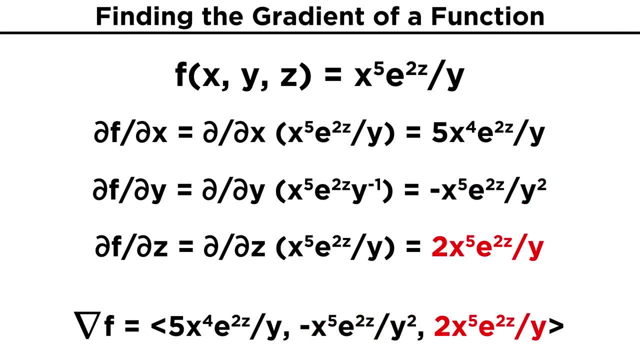 E to the two Z over Y, squared, two X to the fifth E to the two Z over Y as the gradient vector for this function. You may have noticed during this lesson that we have been using our variables X, Y and.